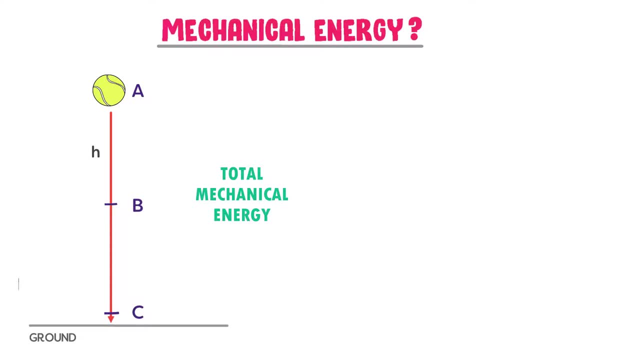 the total mechanical energy of this ball at point A, point B and point C as the ball falls down. Note it down that total mechanical energy is equal to potential energy plus kinetic energy. Let me repeat it: Total mechanical energy is equal to potential energy plus kinetic energy. 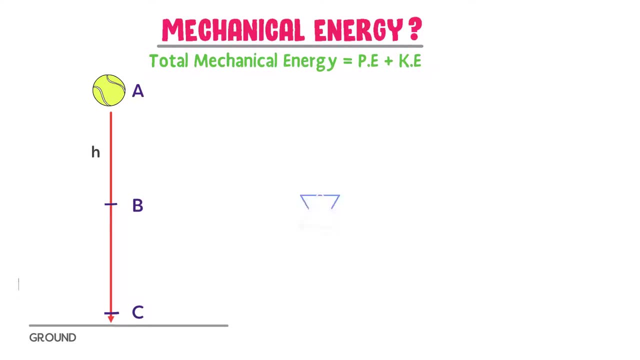 I will often use this equation throughout this lecture. We know that the height of the ball from the ground is h at point A. Let's consider that when this ball reaches to the point B, its height from the ground will be x. What about the height of A? 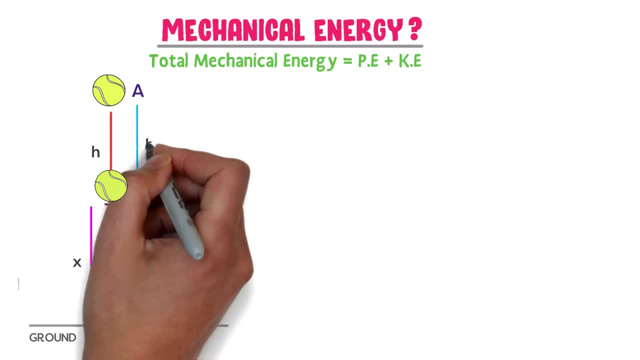 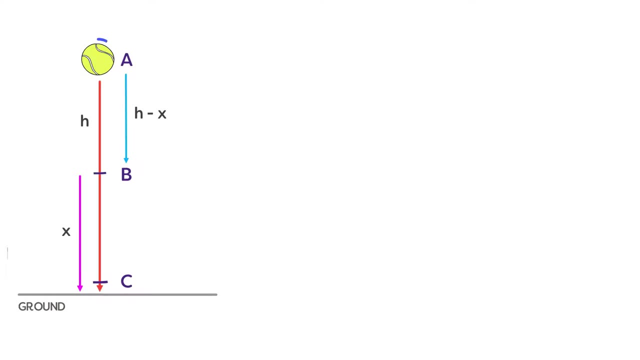 from the point B. Well, it becomes h minus x. Firstly, I am going to find the total mechanical energy of this ball at point A. We know that potential energy is equal to. potential energy of the ball at point A is equal to mgh, where m is the mass of the ball, g is the gravitational. 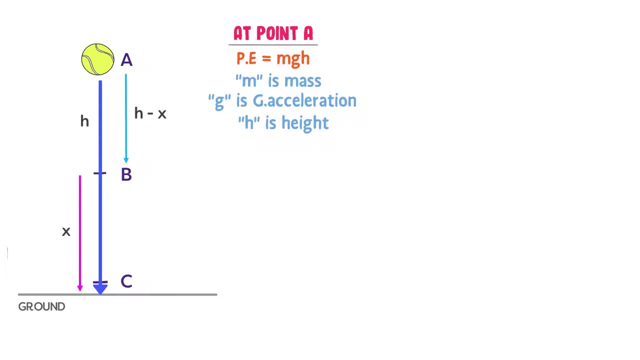 acceleration and h is the vertical height of the ball from the ground. What about the kinetic energy of the ball at point A? Well, we know that kinetic energy is equal to half of mv squared, where m is the mass of the ball and v is the 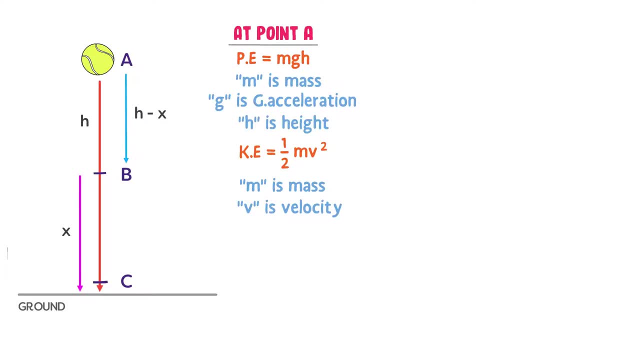 speed or velocity of this ball. We also know that the ball is at rest at point A. Its initial velocity vi is zero. So kinetic energy of the ball at point A is zero because the ball is stationary. We know that total mechanical energy is equal to potential energy plus kinetic energy At point A. 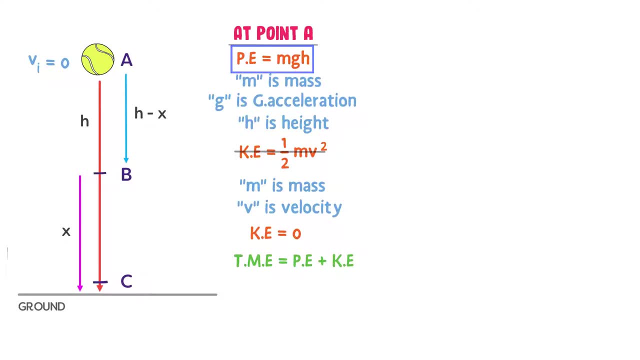 potential energy of the ball is mgh, where m is the mass of the ball from the ground And kinetic energy of the ball is zero. So total mechanical energy at point A is equal to mgh plus zero. Our total mechanical energy is equal to mgh. Thus the total energy of the ball at point A is: 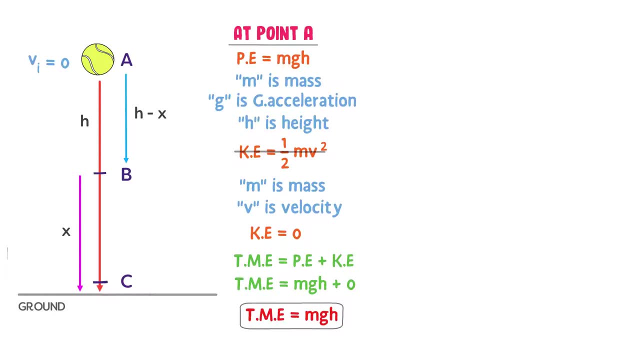 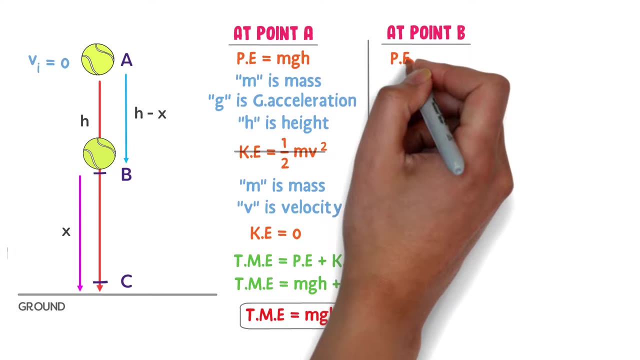 equal to mgh. Now what about the total mechanical energy of the ball at point B? Well, we know that potential energy is equal to mgh, but here, at point B, the ball is present at a height of x above the ground. So we write: potential energy of the ball at point B is equal to mgh. We 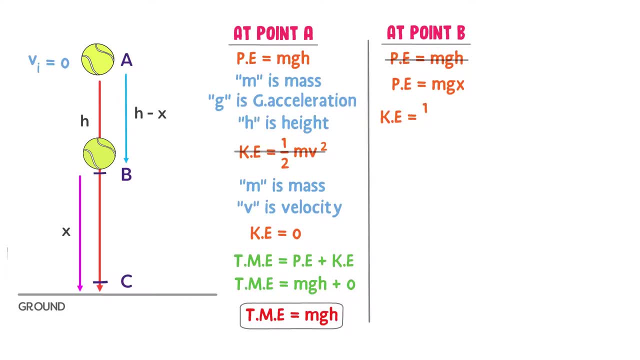 also know that kinetic energy is equal to half of mv squared. Let I call this equation no 1.. Now, Now we can find the velocity of this ball by using second equation of motion, which is: vf squared is equal to vi squared plus 2 gs. 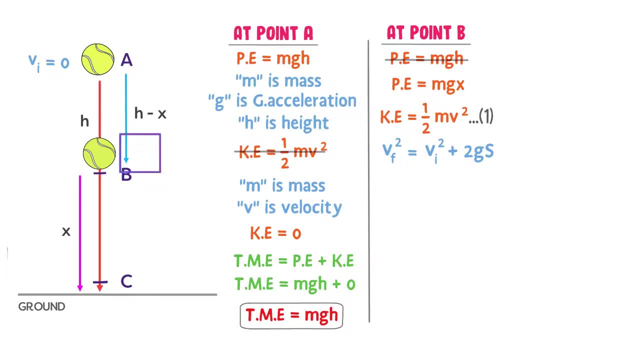 Here, vf is the velocity or speed of the ball at point B, Vi is the initial velocity of the ball at point A And s is the distance the ball travelled from point A to the point B. The initial velocity of the ball is 0.. 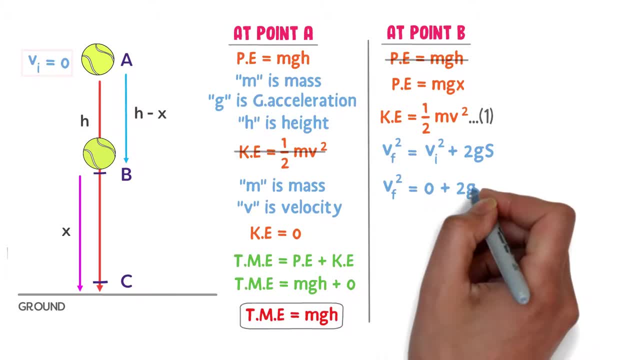 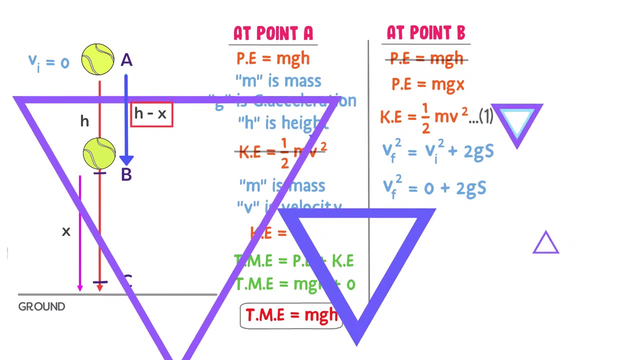 So we write: vf squared is equal to 0 plus 2 gs. We know that s becomes h minus x. Our s is the distance h minus x, which ball travelled while falling down from point A to point B. So we get vf squared is equal to 0 plus 2 g into h minus x. 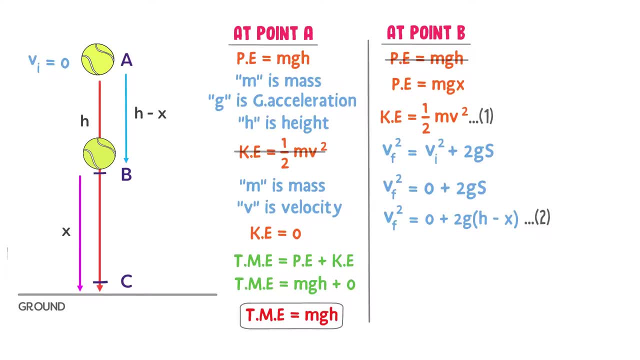 Let I call this equation number 2.. I will put the value of equation number 2 or the value of velocity instead of this v squared and equation number 1.. I get kinetic energy is equal to half of m into 2 g, into h minus x. 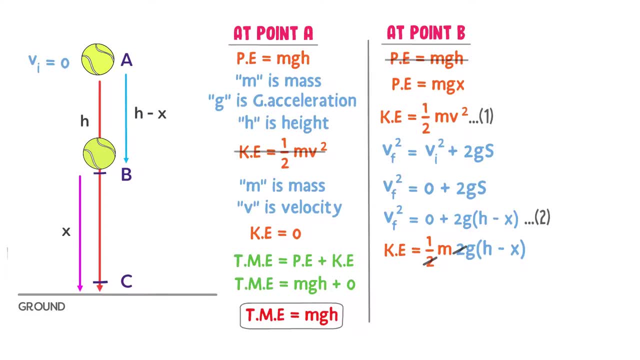 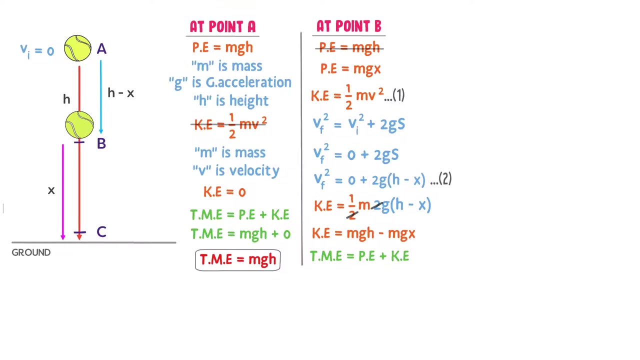 This 2 and this 2 is cancelled out. I get. kinetic energy is equal to mgh minus mg. We know that the potential energy of the ball is mgx and the kinetic energy of the ball is mgh minus mgx. Also, we know that total mechanical energy is equal to potential energy plus kinetic energy. 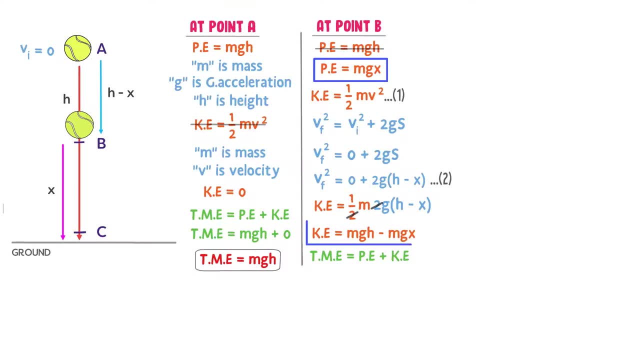 So I put the value of potential energy and kinetic energy in this equation. I get: total mechanical energy is equal to mgx Plus mgh minus mgx. This positive mgx and this negative mgx cancel out, I get total mechanical energy is equal to mgh. 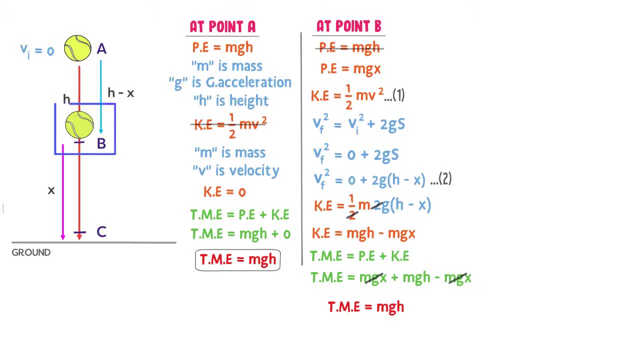 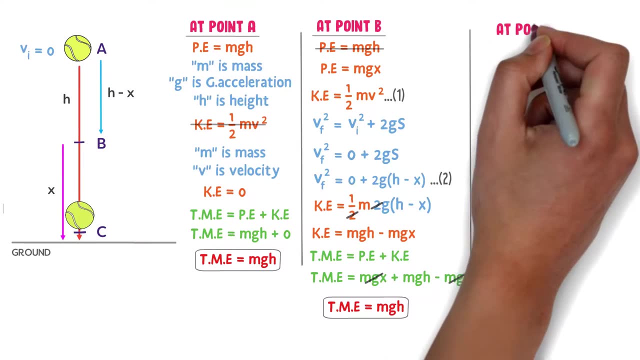 So the total mechanical energy of the ball at point B is also mgx. Now, what about the total mechanical energy of the ball at point C? Well, note it down that at point C the ball doesn't touch. So we know that it doesn't touch. 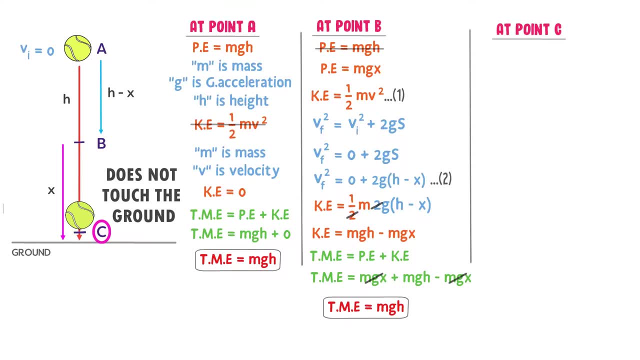 So we know that it doesn't touch. So we know that it doesn't touch the ground. It is slightly above the ground or we can find the total mechanical energy of the ball at point C, just before hitting the ground. We know that when the vertical height of the ball 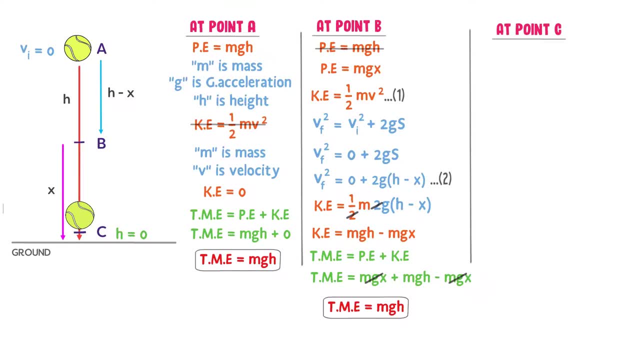 becomes zero, its potential energy also becomes zero. Hence, potential energy of the ball at point C is zero. What about its kinetic energy? Well, we know that kinetic energy is equal to half of mv squared. Let I call this equation number one. We find the velocity of the ball at point C again. 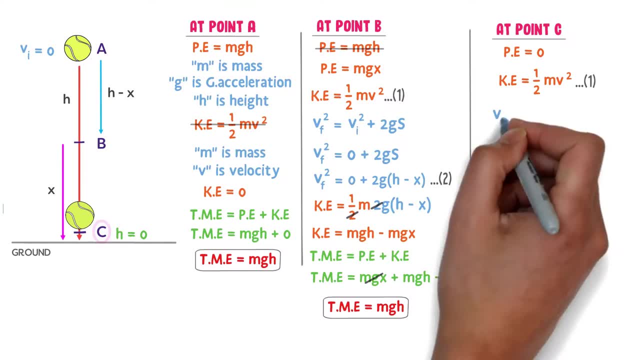 using second equation of motion, which is: vf squared is equal to vi squared plus 2gs. The initial velocity of the ball is zero, So we get 0.. vf squared is equal to zero plus 2gs. We know that here s becomes h, because s is the distance. 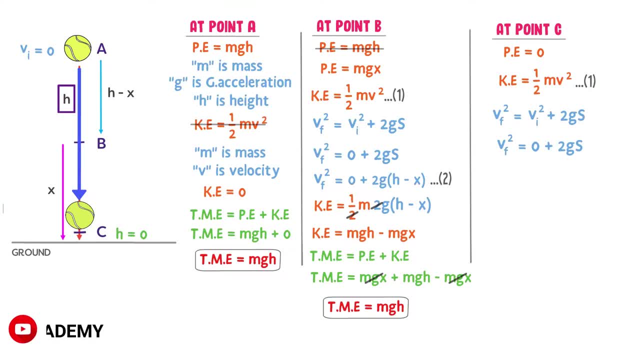 which the ball travels from point A to point C and the ball travels h times distance. So I get vf squared is equal to 2gh. Let I call this equation number two. Now I will put the value of velocity …. I get: kinetic energy is equal to half and to m and to 2gh. This two and this two White. 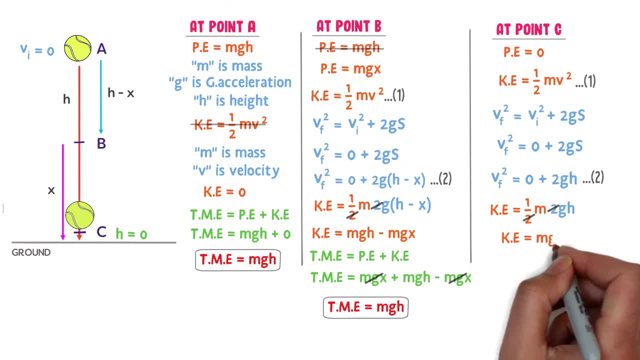 Layout presents an interesting equation. So the positive energy of the guy at point C and the crazy guy at point C have been equal to m and to 2gh. I get, kinetic energy is equal to m and to 2gh同. They are different values of energy in terms of momentum, Since teeth are fixed at point.